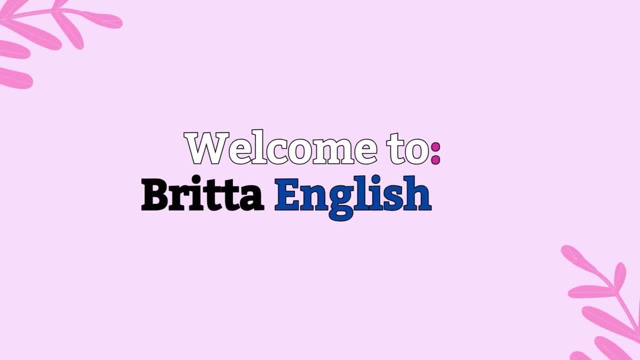 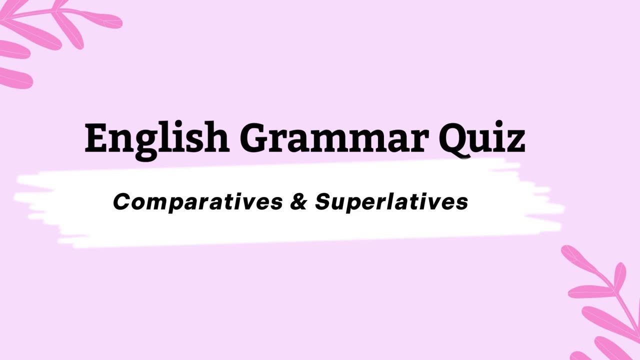 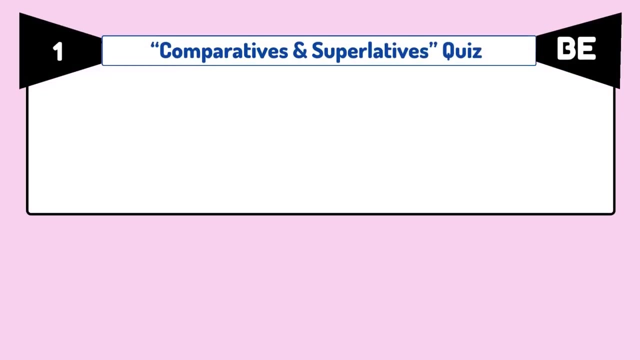 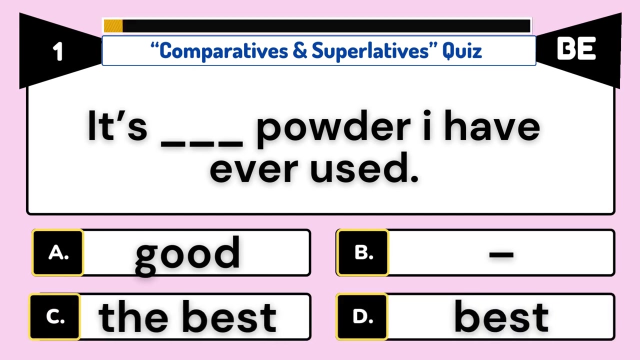 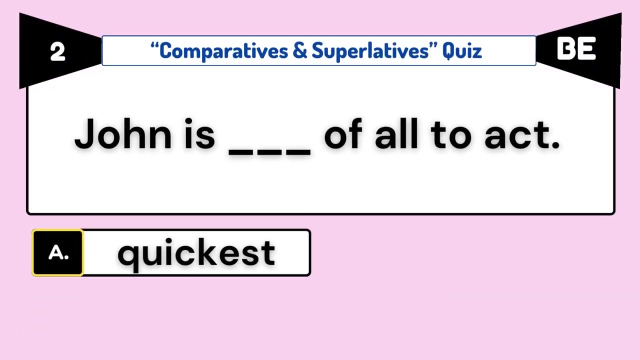 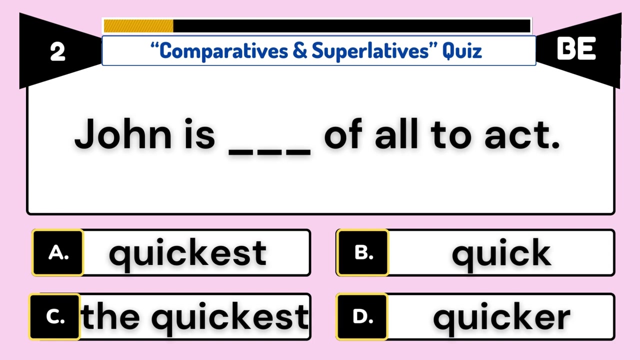 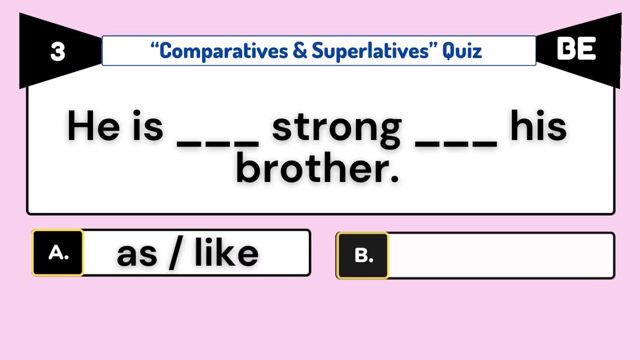 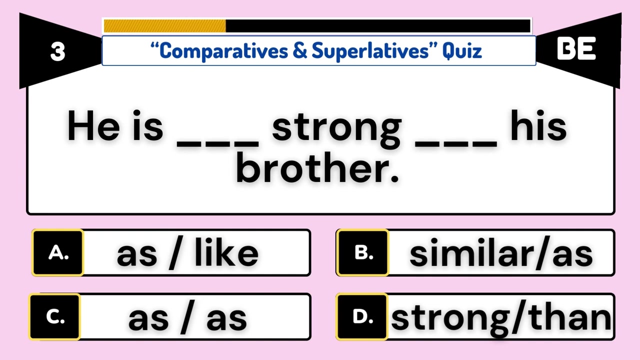 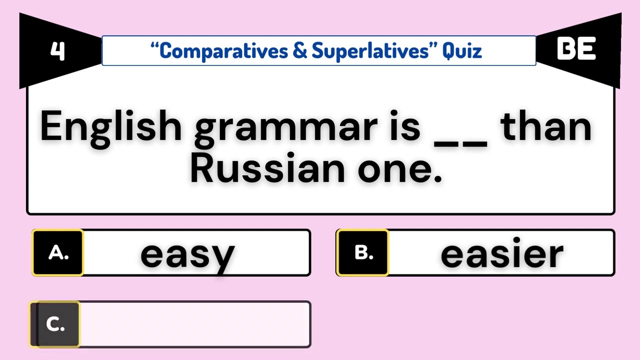 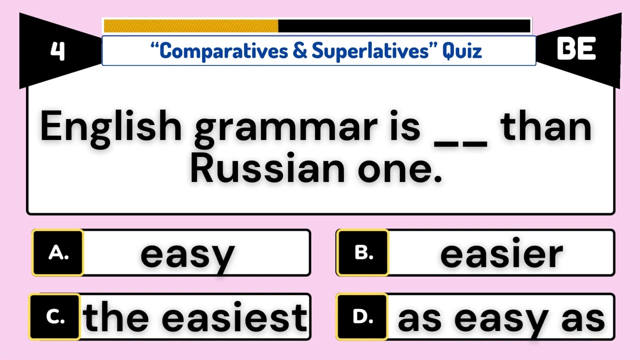 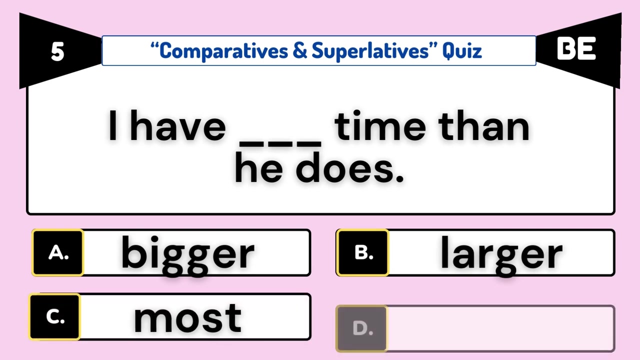 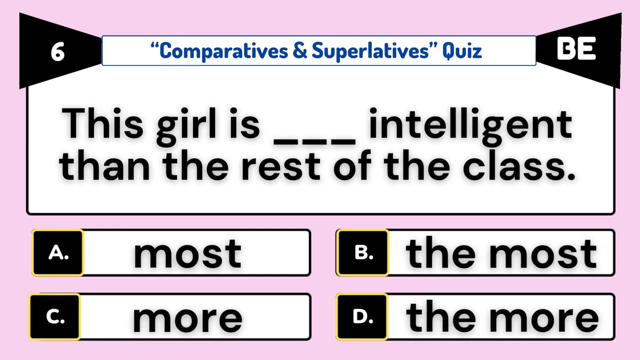 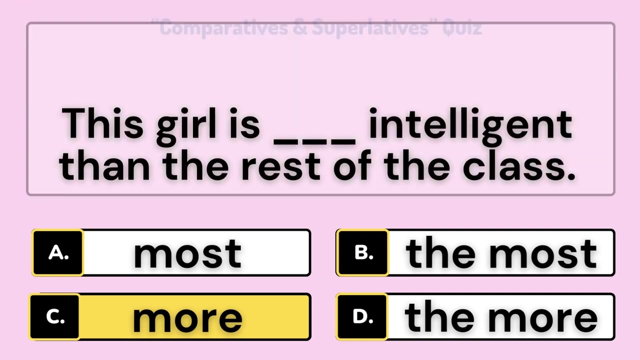 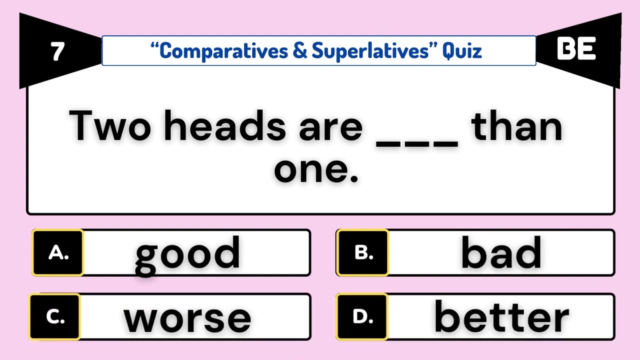 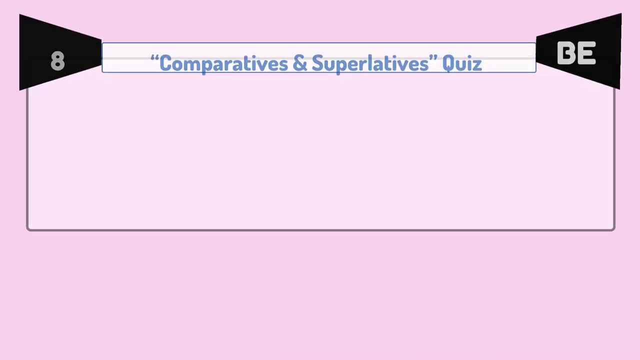 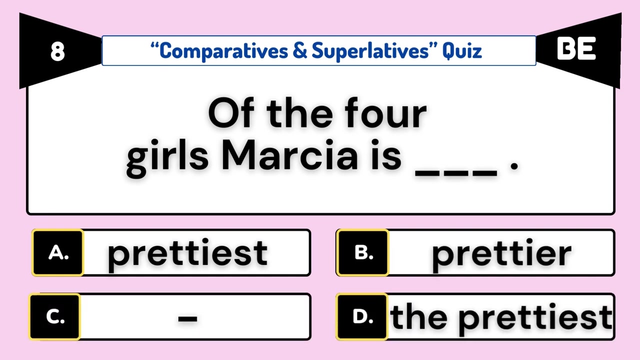 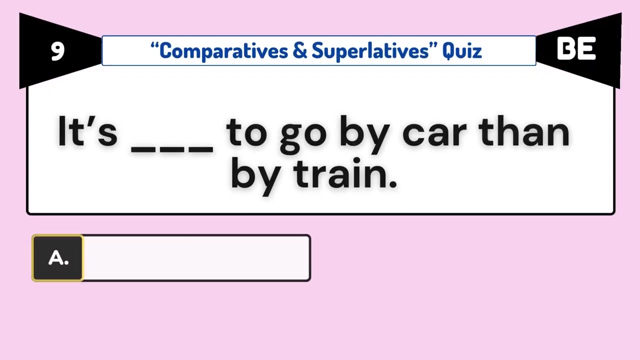 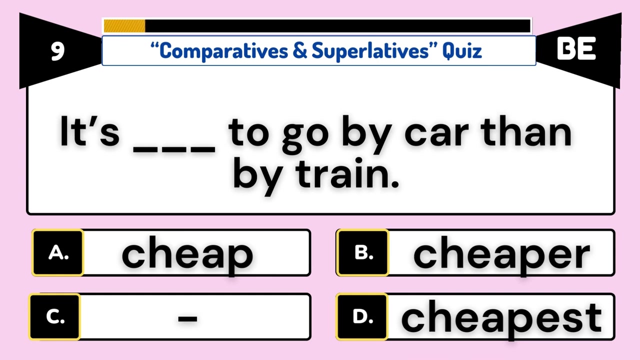 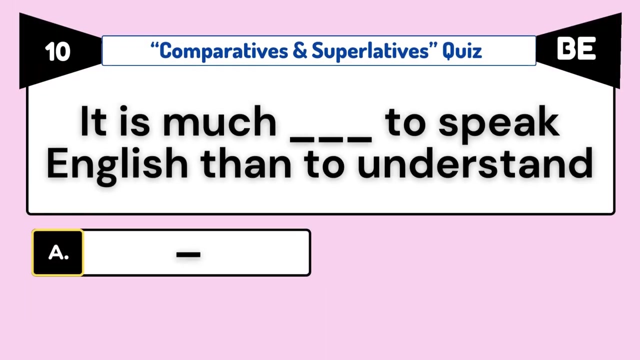 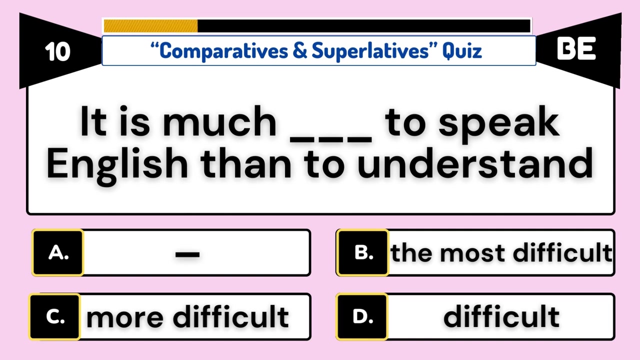 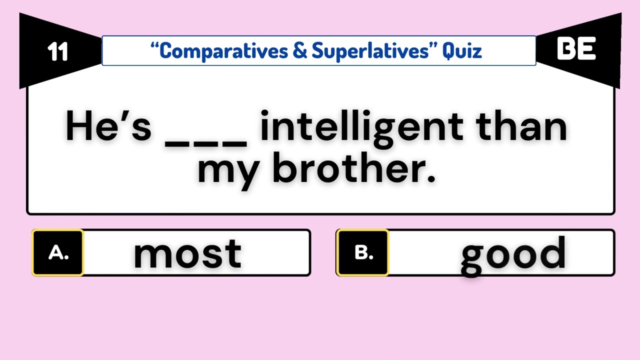 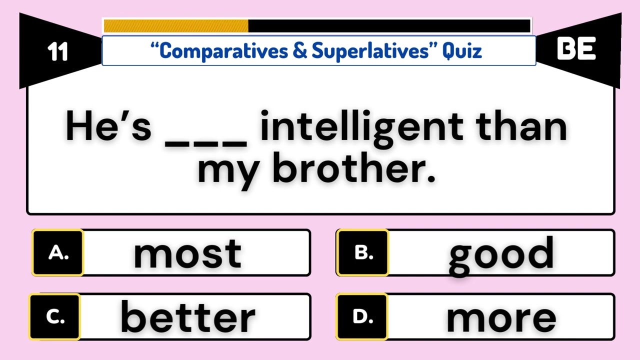 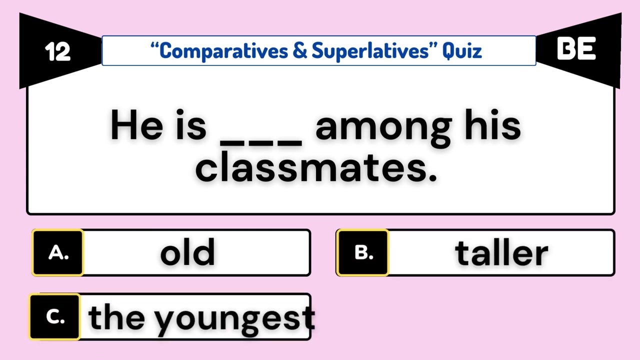 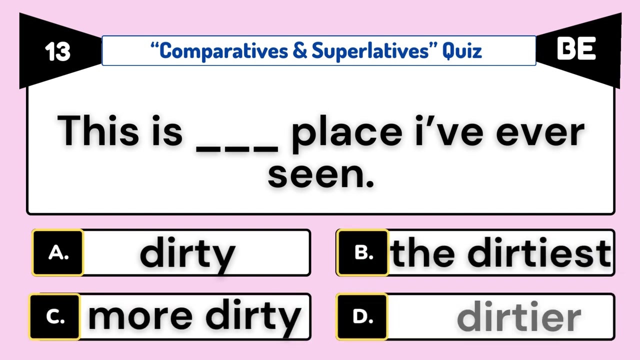 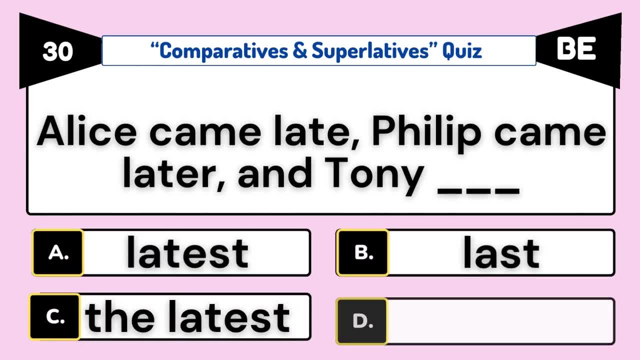 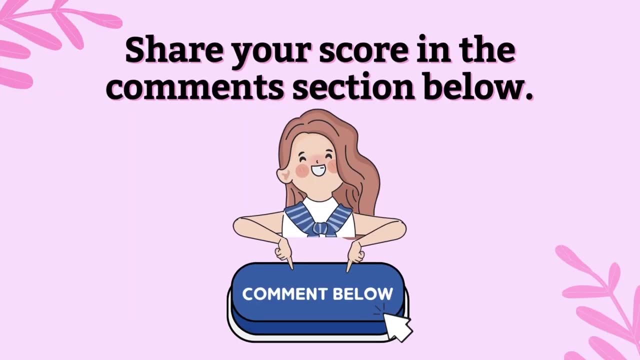 How many questions did you get correctly? Share your score in the comments section below. 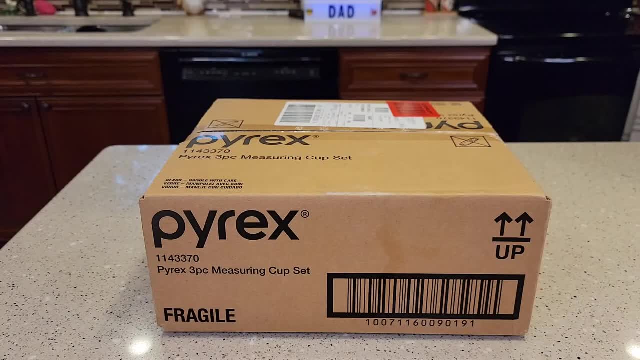 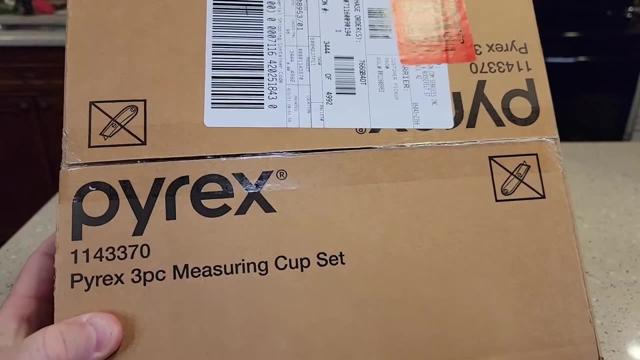 Hello everyone, this is Just a Dad. Today I'm going to do an unboxing and review on this Pyrex glass measuring cup set, the three-piece set. It comes with a one cup, two cup and four cup. So the first thing it says: don't use a utility knife. 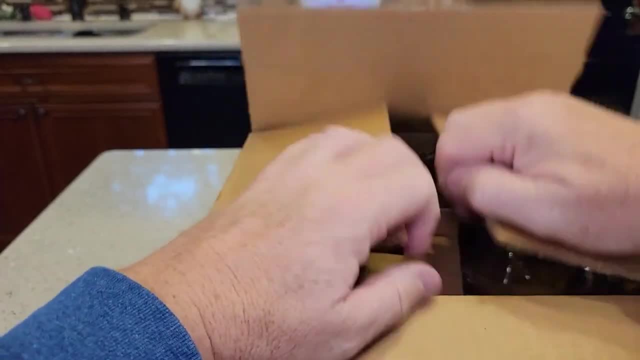 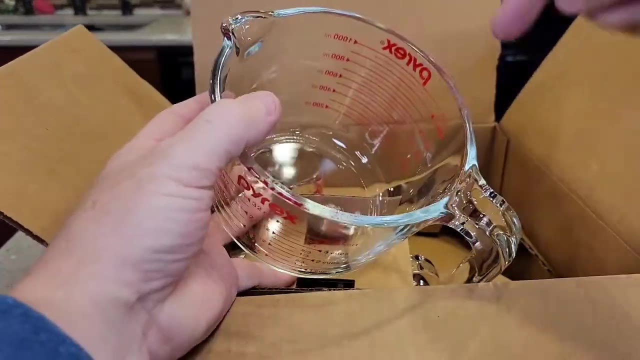 So I'm not sure. maybe they're afraid you'll cut through. You could nick this glass and that might cause it. yeah, So I definitely wouldn't stick a utility knife way in there. you could definitely nick these. So this is a big box. 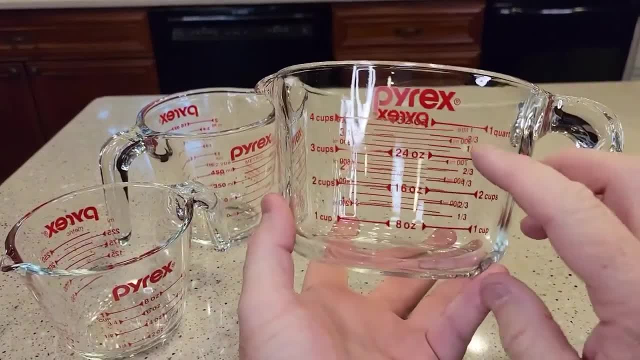 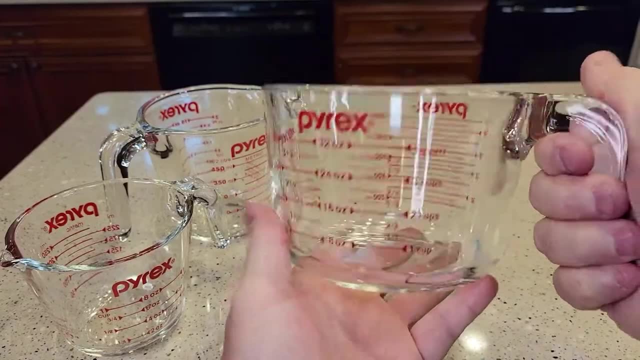 So these are kind of heavy duty. this one's a little bit bigger than I thought: One quart, four cups. it's very thick. I really like the handle. it's all glass. It says it's microwave and oven safe. But the reason I got it, I like all the measurements. 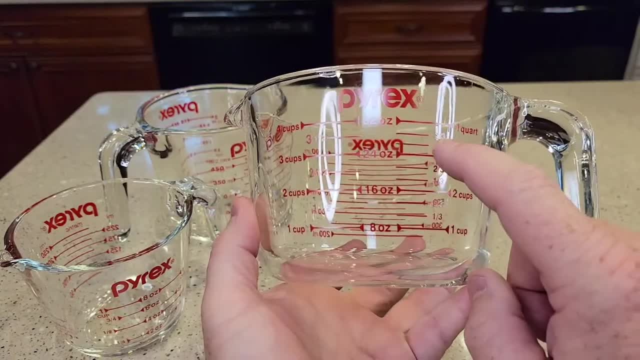 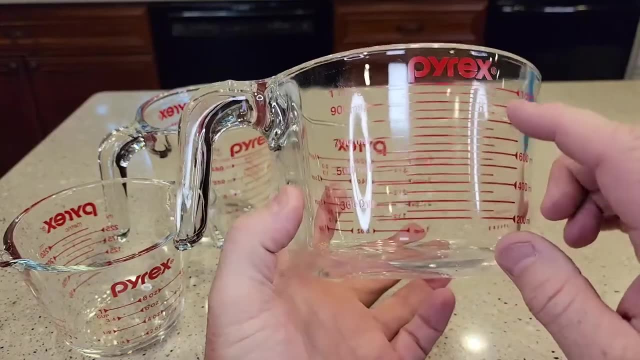 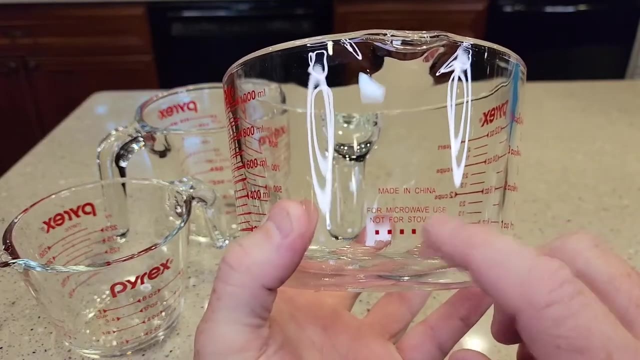 I want ounces, quarts, cups, even two-thirds of a quart. What do we got on the other side? Then we got milliliters And liters, Very easy to see. I like that For microwave use, not for stovetop. 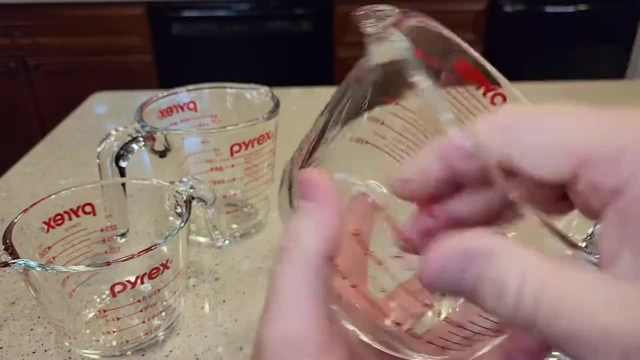 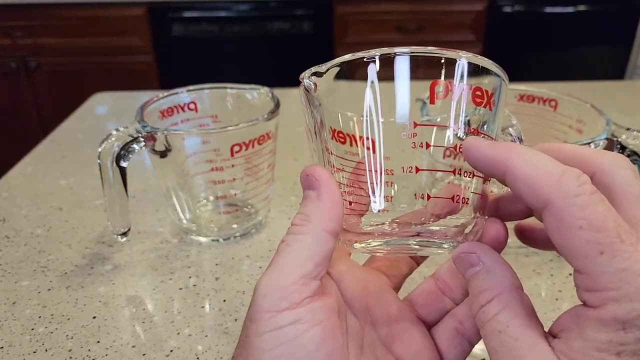 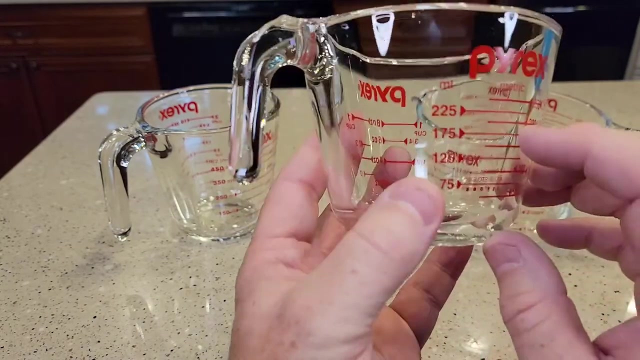 Okay, so bottom of it seems very flat and it pours. Really I want this one. This is the one cup eight ounce, one cup Milliliters 250, and it's got kind of an in-between on this one. 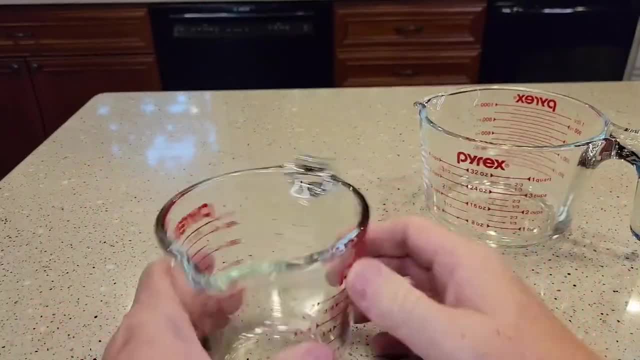 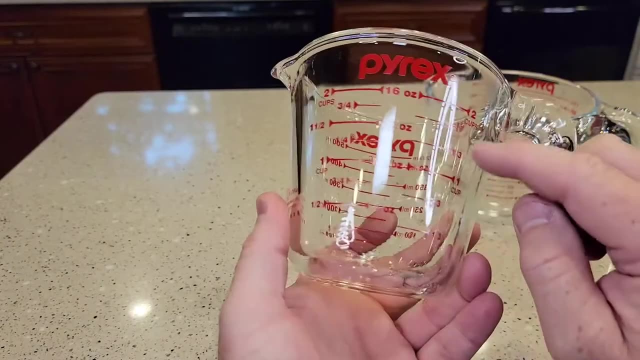 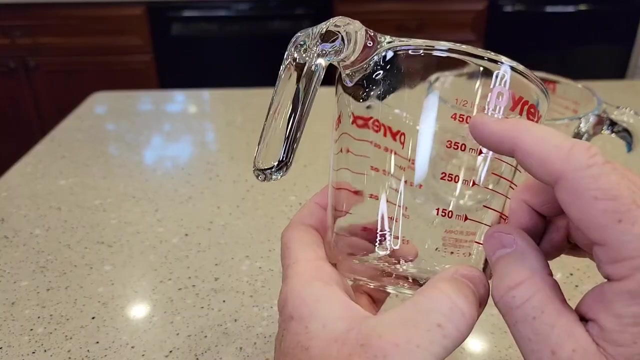 This one feels real nice and this is the pretty common two-cup, Two-cup ounces, cups, cups. looks like it's got the same cups on it. Then we got 500 milliliters to 100, and half liters.